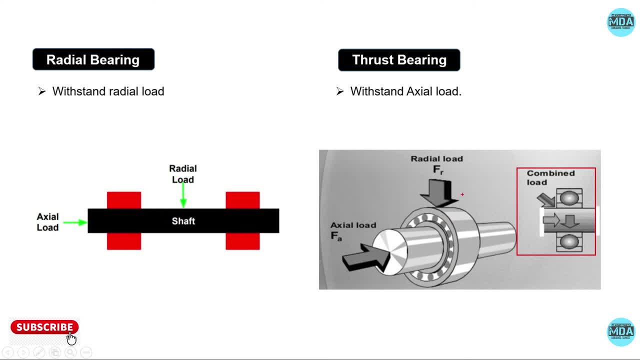 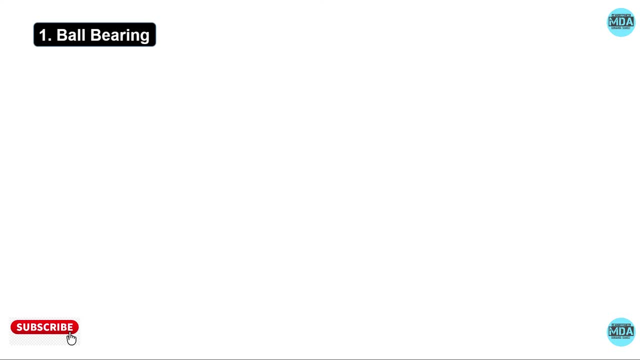 axle and and the radial load. the ball bearing is a commonly used types of bearing and it used to handle the both radial and the thrust load. the various types of ball bearings are available in the market. the first one is the single row ball bearing. in that type of a single row ball bearings, the balls are arranged in a 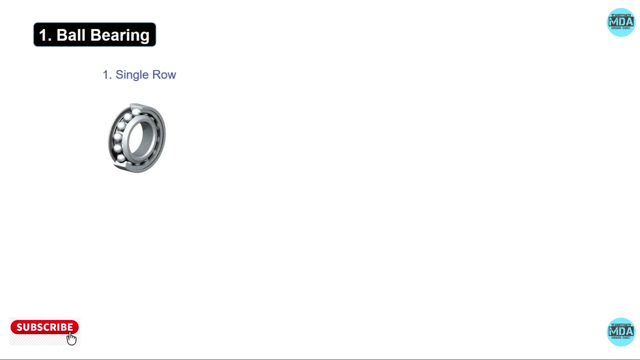 single row and they are used to handle the radial loads. double row ball bearings. so in that the balls are arranged in a two rows and compared to single row ball bearing, double row ball bearing have more load carrying capacity. deep groove ball bearing. so these types of ball bearing are used at. 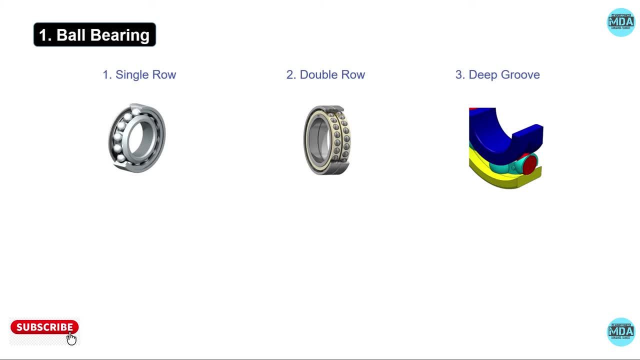 very high rotational speed because it offers low friction, low noise and the low vibration. so next one is a angular contact ball bearing. so in these types of bearing the inner and outer ring are in contact with the ball at an angle, so it can. it can take both the radial and the 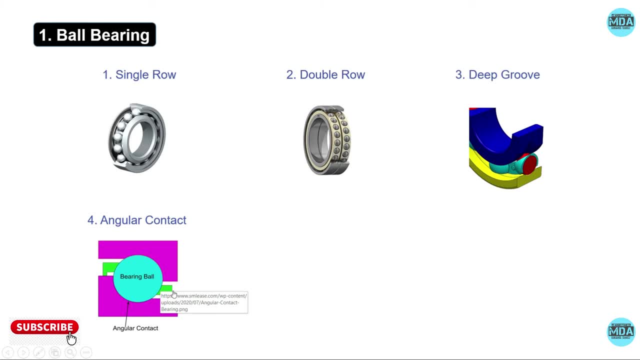 axial load. simultaneously, the load carrying capacity of load carrying capacity of the bearing depends on the load carrying capacity of the bearing. and the load carrying capacity of the bearing depends upon the ball and the ring contact angle. next one: we have the self aligning ball bearing. so these types of ball bearing are used where the angular misalignment of the shaft with 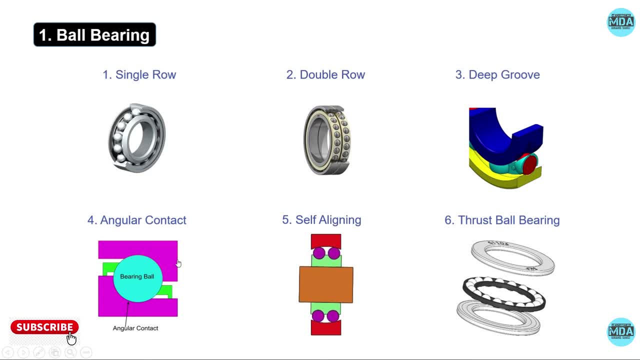 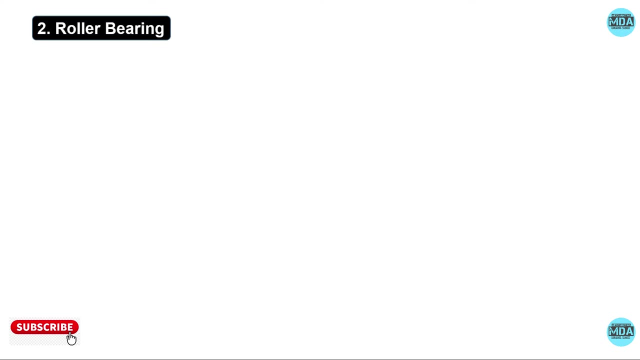 the housing. next one: we have the thrust ball bearing. so these are used to handle the axial load only so and it is available in a single and a double direction bearing. next one is a roller bearing. in a roller bearing instead of ball, we use here roller to support the 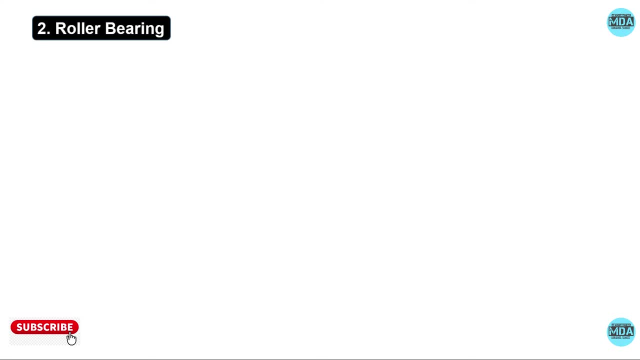 rotating shaft. so roller can provide the large contact area compared to the ball bearing to bear their high load capacity. so the roller bearings are used in a power generation unit, wind turbine unit, gear drives and machine and the gear reduction unit. so the various types of the roller bearings are available in the ball bearing. so these types of ball bearings are used in a 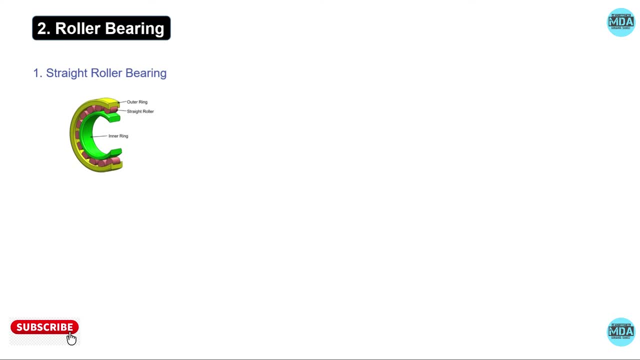 market. so let's discuss one by one. first one is a straight roller bearing, in that the cylindrical roller handle the thrust coming from the housing. tapered roller bearing: in these types of bearing the rollers are arranged at an angle so the tapered roller bearing can handle the axial and 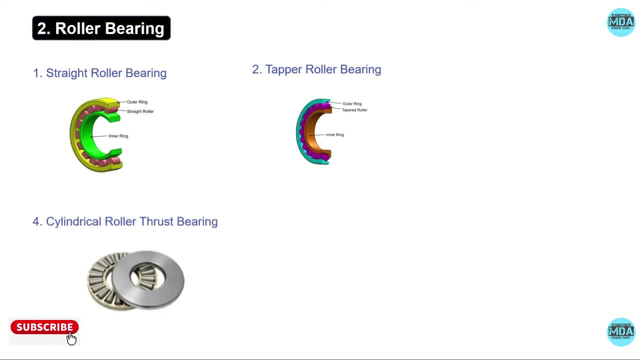 the radial load force cylindrical roller thrust bearing. so these types of bearing will handle only axial load. next one is the spherical roller bearing. in a spherical roller bearing the inner ring with the two raceway at an angle, and they are used to handle the heavy radial and the axial load general and sliding bearings. 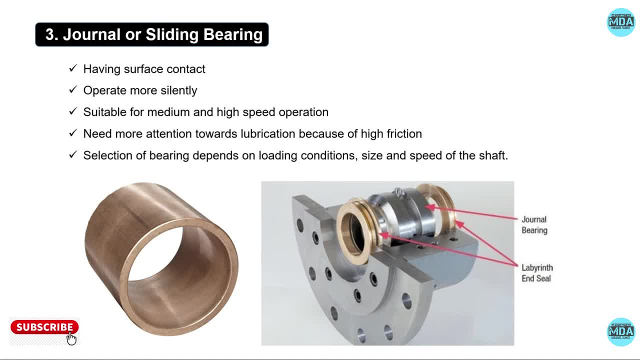 these types of bearings have the largest surface contact and large frictional. these types of bearing will operate more silently and these type of bearings are suitable for medium and high speed operations. so here the attention toward the load is very important, so the bearing is very important, lubrication is very important because of here more friction, here the selection of the bearing, it. 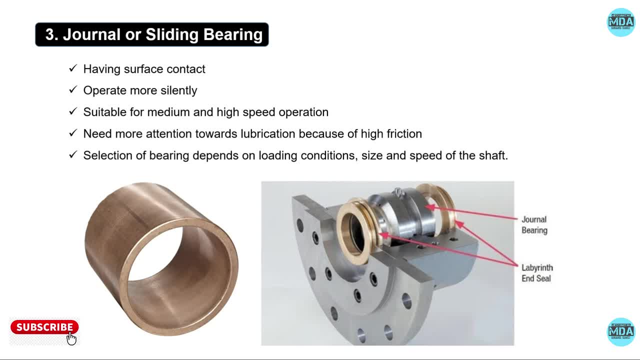 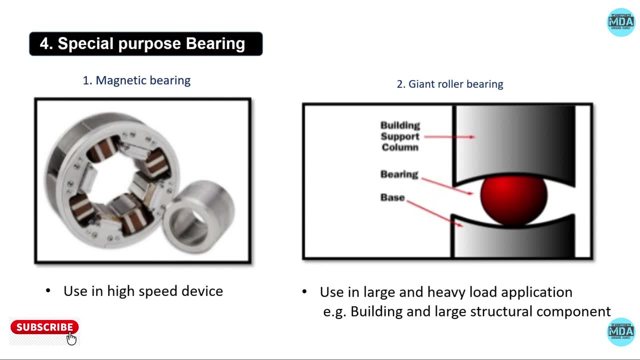 depends on the size, load condition and the speed of the shop. some special purpose bearings are magnetic bearings and the grand roller bearings. magnetic types of bearings are used in high speed devices. in these types of bearing there is no, no moving parts. and next one is the gland roller. 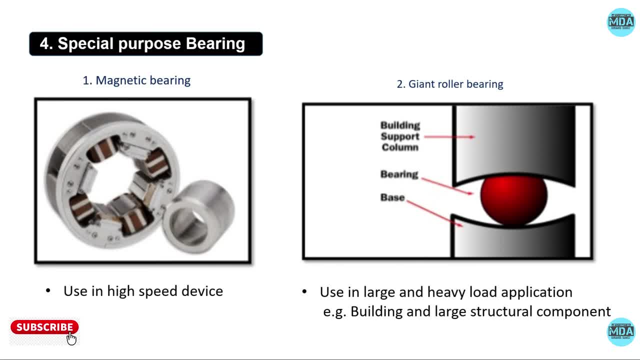 bearing. these types of bearing are used in the large and heavy load application. these types of You can see in the building's large structure component bridges. 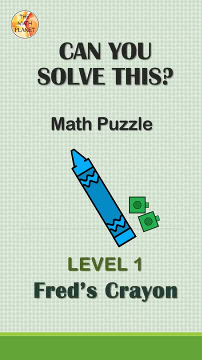 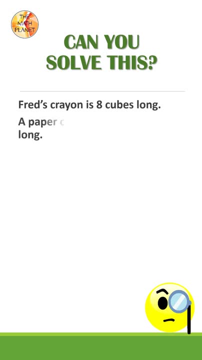 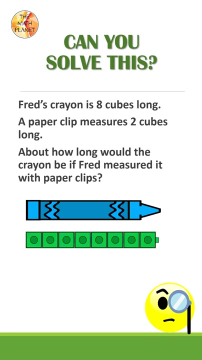 Can you solve this? Level 1. Fred's crayon. Fred's crayon is 8 cubes long. A paper clip measures 2 cubes long. About how long would the crayon be if Fred measured it with paper clips? Level 2. We will draw a picture to solve. Fred's crayon measures 8 cubes long. If the paper clip has the length of 2 cubes, the crayon's length will be about 1,, 2,, 3,, 4.. The crayon is 4 paper clips long.